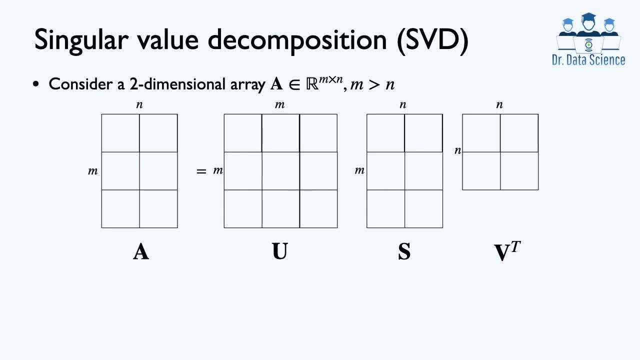 So, to summarize, we assume that a has m rows and n columns And in this decomposition we see that u has m rows and columns, S has m rows and n columns and the matrix v has n rows and n columns. This means that both matrices u and v are square matrices and s is rectangular. 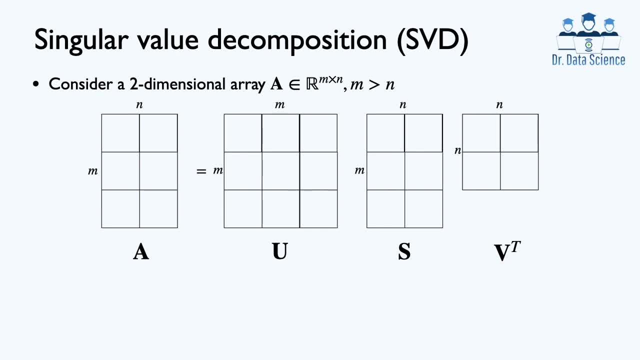 Now I explain these three matrices individually to understand their properties. The columns of the matrix u are called the left singular matrix. The columns of the matrix u are called the left singular matrix. The columns of the matrix u are called the left singular matrix. 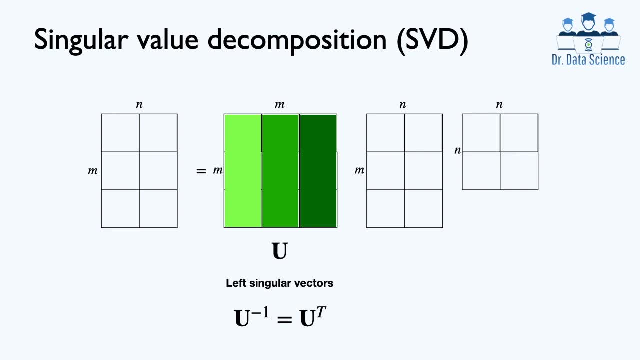 And the matrix u is orthogonal And the matrix u is orthogonal, Which means that the inverse of matrix u, u inverse, is equal to transpose of u, which we show here by u transpose. This is a really useful property because we know that finding matrix inversion is difficult in general. 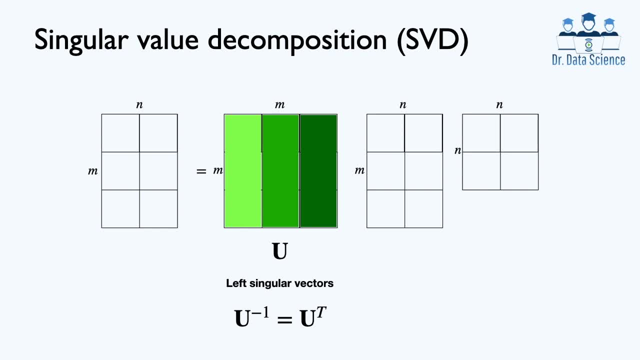 And in this special case, we can simply transpose the matrix into a singular matrix, which is a singular vector, Which means that we have one singular vector to find its inverse. Now let's take a look at the matrix V. The columns of V. 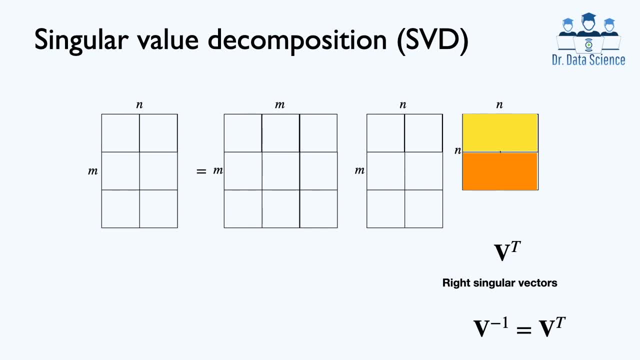 which they correspond to. the rows of the matrix V transpose, as we color coded here are called the right-singular vectors, And V is also an orthogonal matrix, which means that the inverse of matrix V is is equal to its transpose. So in that sense matrix V is very much similar to U that we saw in the 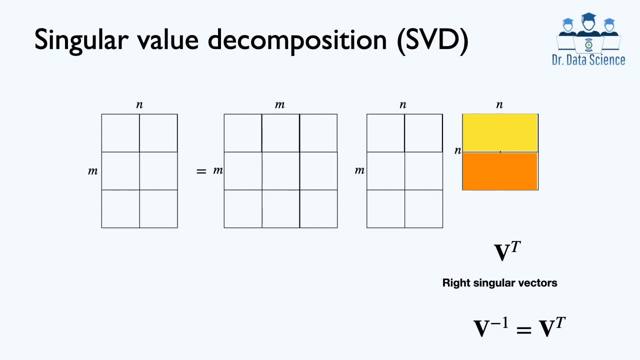 previous slide. In my opinion, the most interesting and important part of computing SVD, or singular value decomposition, is to analyze the matrix S. in the middle, The diagonal entries of S are called singular values and all remaining entries, all the off-diagonal elements, are all zeros. 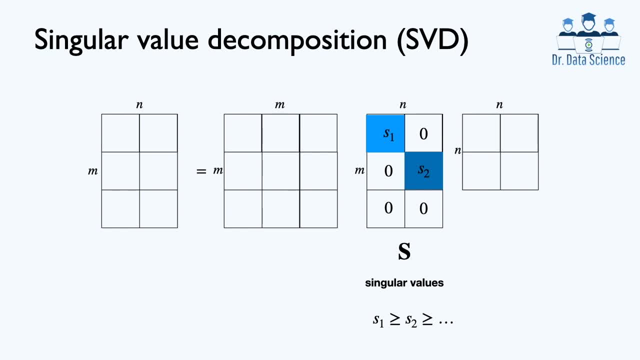 Here we call the diagonal elements S1 and S2.. And one thing that is extremely important to remember is that we sort these singular values in non-increasing order. So let's take a look at the matrix V, which is the right-singular vector, and we sort these singular values in non-increasing order. And one thing that is extremely important to remember is that we sort these singular values in non-increasing order. 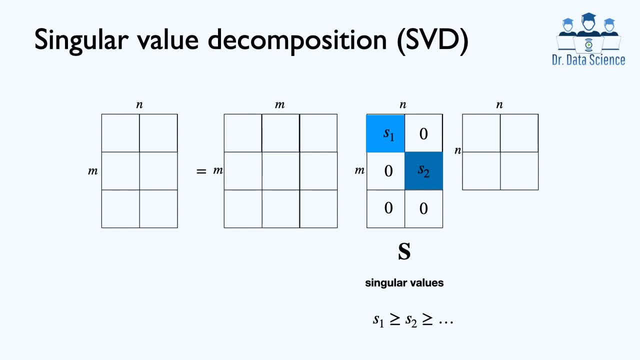 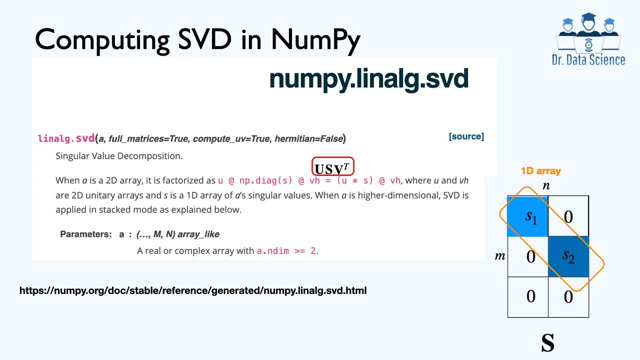 So this means that S1 is greater than or equal to S2, and similarly, if we have more singular values, So they are sorted in non-increasing order, So the bigger one is first one and then we have smaller singular values. So, in order to compute SVD in NumPy a, 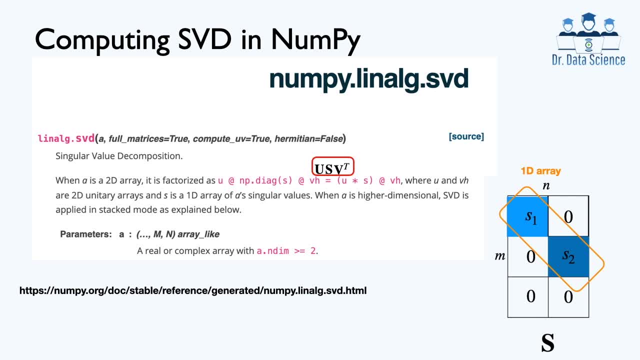 where we use for computing with arrays, there is this module called lin-alc or linear algebra, And we can use lin-alcsvd And the first input argument is the input array that we have and mostly we work with two-dimensional arrays like the one: 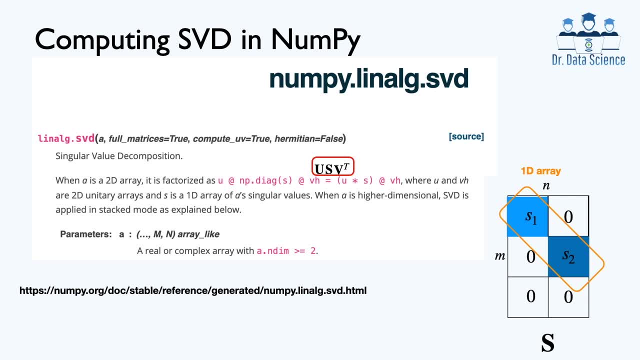 we saw the matrix A And that means that we have to give that matrix A to these built-in function, And the way that it works is summarized in the documentation page. So this function gives us the matrix U and also the matrix V, And then the only thing that is very important: 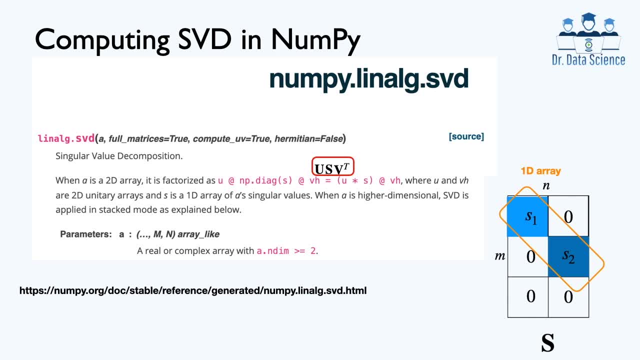 here to remember is that because the matrix S that we talked about in the previous slide is always diagonal, meaning that all the elements on the main diagonal are these singular values and all the off-diagonal elements are zeros, we can simply just store the diagonal elements. 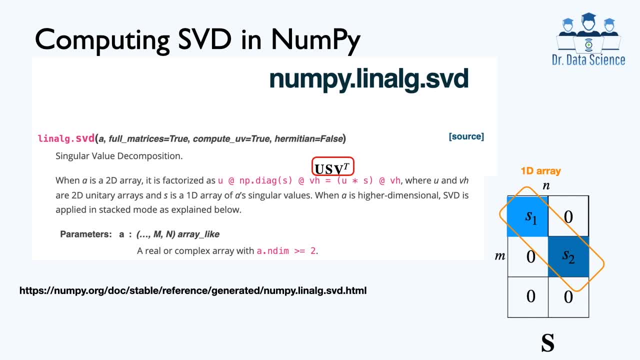 as a one-dimensional array And then, whenever you want to construct this matrix S in this form that we have, in this two-dimensional form, then you can use npdag. So npdag takes a one-dimensional array and puts those elements on the main diagonal and then we will have. 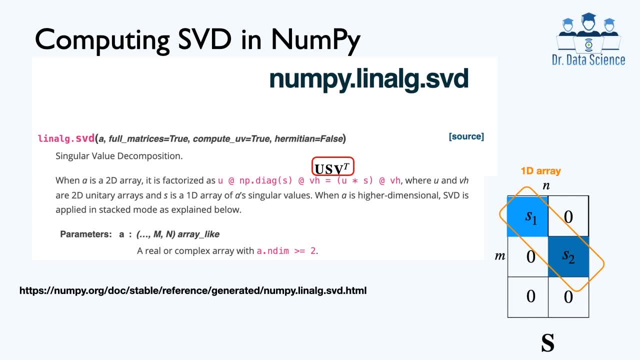 zero padding in all other entries of these metrics. So if you are interested, you can go to this page and see more about singular value decomposition in NumPy. But I summarized the main points here, And another important option that we have here is this: 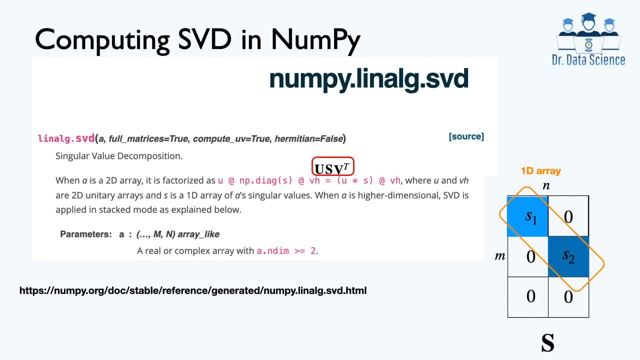 thing that is called full underscore matrices. that by default is true and we can set these also to be false. So the difference is that if you look at this matrix S, here, the third row, we have zero and zero, which means that there is nothing really useful in that row. 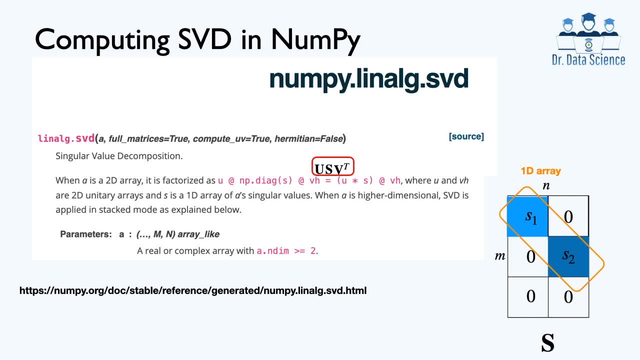 of these metrics. So we can just simply have a two-by-two matrix where S1 and S2 are on the main diagonal. So in this case we can get rid of the third row, and similarly we can get rid of the third column of the matrix U, And that happens when you set full matrices to be false. So then, 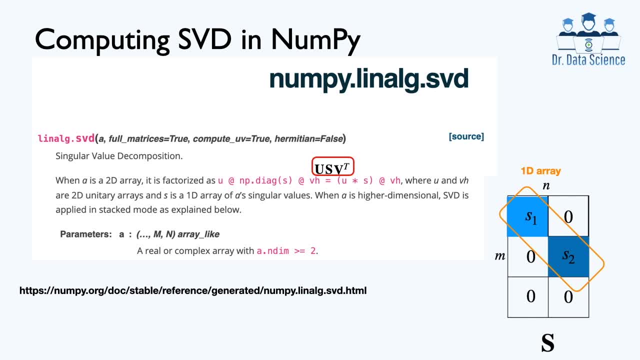 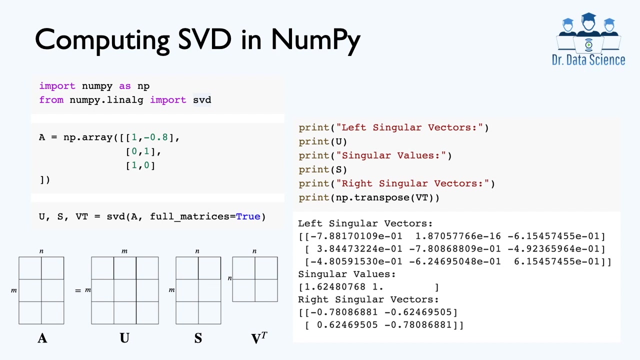 the matrices U and V are not necessarily square matrices, So that's the only difference here. But it can save us a lot of memory storage space, because then you are going to just keep fewer columns and rows in these matrices. So now let's look at this example: We import NumPy as NP and we also import SVD from numpylinalph. 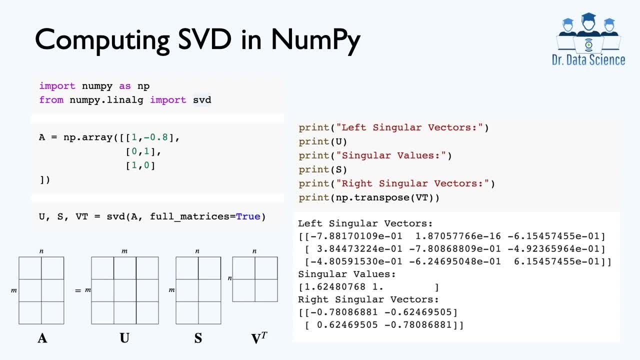 And, by the way, as I promised at the beginning of this video, we will have a full implementation of these에게 at the end of these lectures. lecture notes. So here we create a matrix A that has three rows and two columns, And you can call the function svd, and we set the option for matrices to be true. 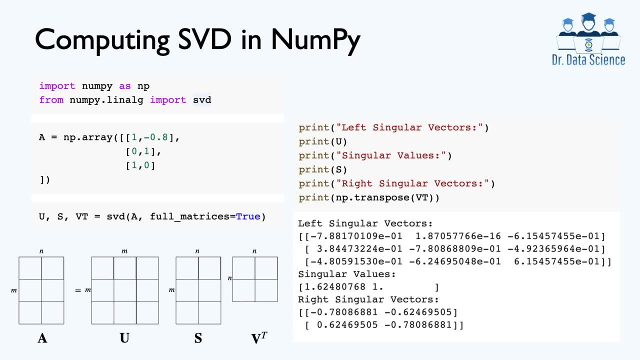 So this will give us square matrices u and b, because it's set to be true, And now we can print u, which contains left-singular vectors, and then the diagonal matrix s. And remember that the s that this function gives us is always a one-dimensional array, which you can 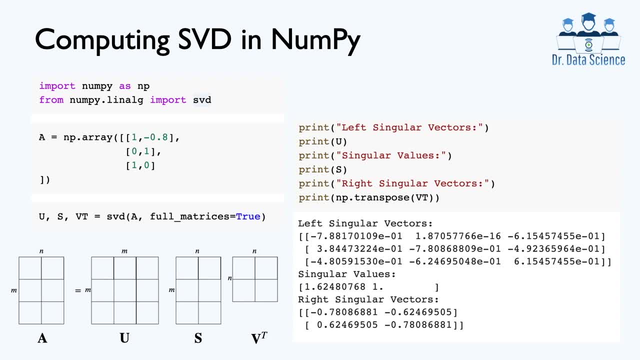 see here that the first element is 1.62 and then the second element is 1.. And, as we said, these things are always in non-increasing order, meaning that the second one here, if you look at it, is 1, which is less than 1.62.. And then for showing the right-singular vectors, because it is common to have 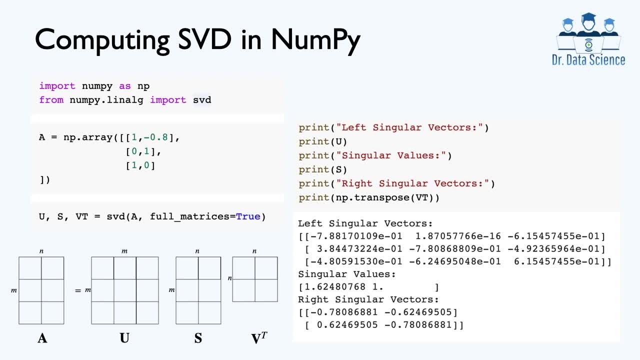 these singular vectors in columns rather than rows. that's why I transpose that matrix that I call vt, because by default this vt- the right-singular vectors- are in the rows, And then if you want to have these in columns, you can just call the transpose, and now we can have them in the right. 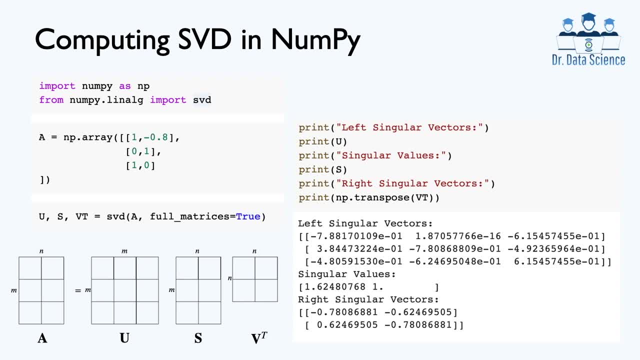 format, But this really depends on the notation. So some textbooks, for example, they have row vectors. some textbooks they have column vectors and it is more common to have these left and right-singular vectors in columns rather than rows. So now, using those right and left-singular vectors, we can see that the right-singular vectors are in the rows. 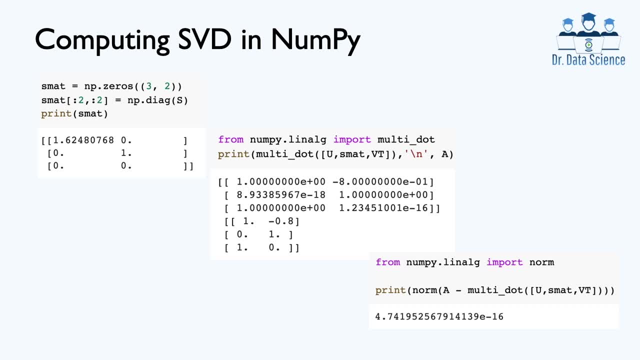 So now this is kind of like create a vernacular and function, but withLEYGEN. Can you remember how popular this was? I think an example of a simple come back method is when you put triggers in a prefix Boolean rule and then you put the variables into the right-singular values and then you put those right-one abilities. 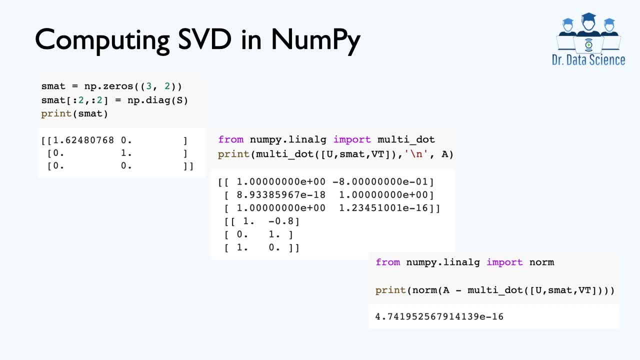 in the arm and you pick what you want to be the right-singular values from that particular function and then you create thestraps And to predict the小 dans into yourером, you are able to do this by having a node s which, if you remember, there were 1.62 and 1 on the main diagonal, and now we have to multiply. 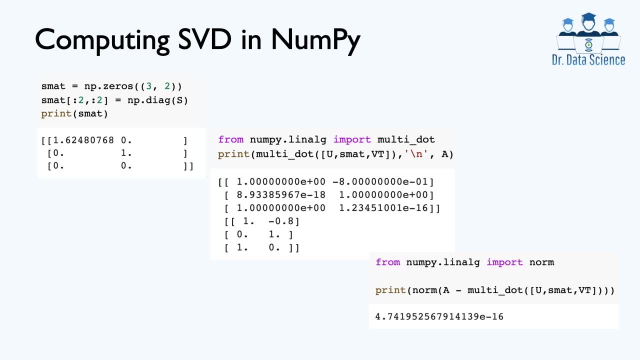 these three matrices, right u and this matrix s in a two-dimensional format, and then vt, which is the which contains the right singular vectors. and in order to do so, we can use again another useful built-in function available from numpylink, which is called multi underscore dot. so in this case you 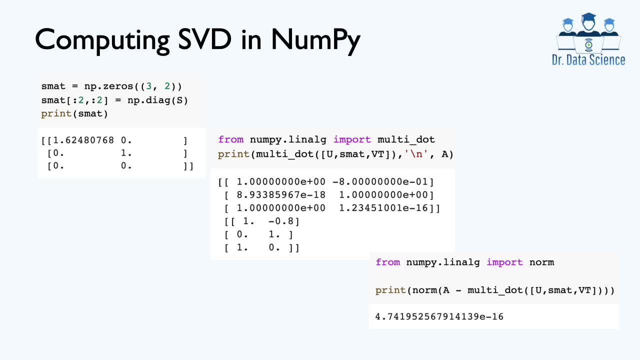 put in one list the all the um functions that you're trying to, all the matrices that you're trying to multiply together in the right order. so we are multiplying u, s and v, transpose, so you can see that here. and if we do so and compare this with the matrix a, we see that they're actually 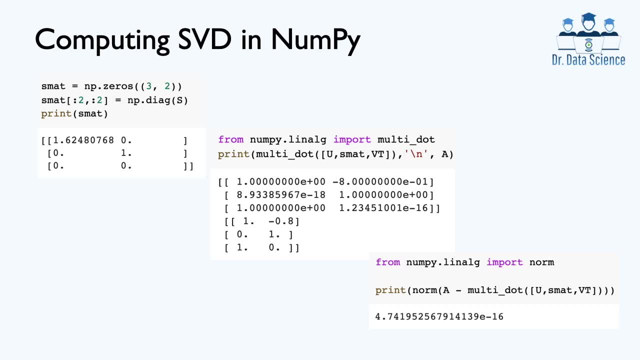 very close. so the first element is one to the power of 10, to the power of zero, that's that e zero. and then we see that we have, um, that negative 0.8, and then we have this e to the power of negative 18, which you know numerically speaking, that's, you know, zero in terms of like. 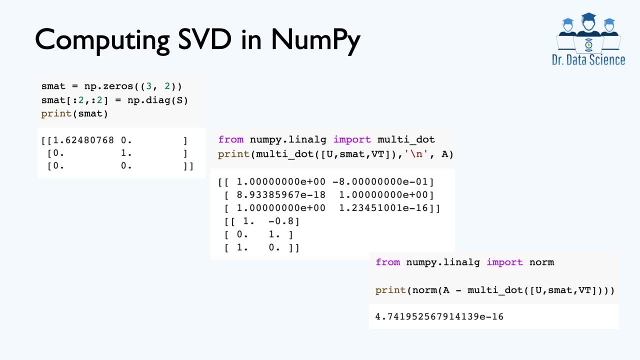 uh, the actual importance of that location. and then similarly for that 10 to the power of negative 16. and if you want to be a little bit more precise, we can do, we can use the norm function from again. lean out and try to find the difference between matrix a and its reconstruction using 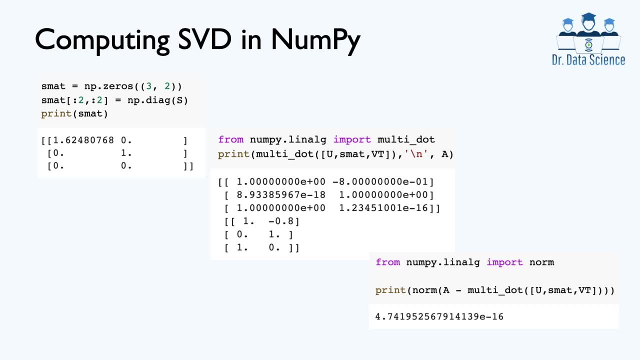 this singular value decomposition, and here we use something called frobenius norm which, after we subtract these two matrices, element wise, we are going to square all those elements, add them together and then take the square root which, as we can see, is something in the order of 10 to the 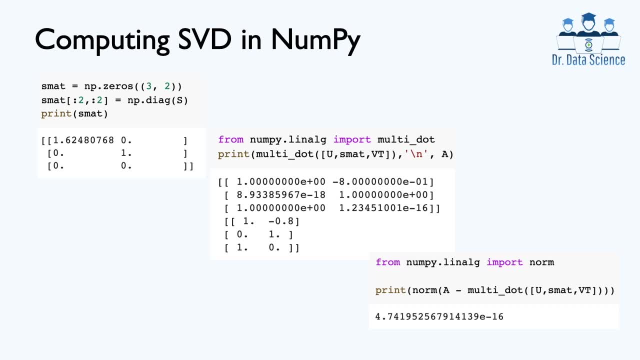 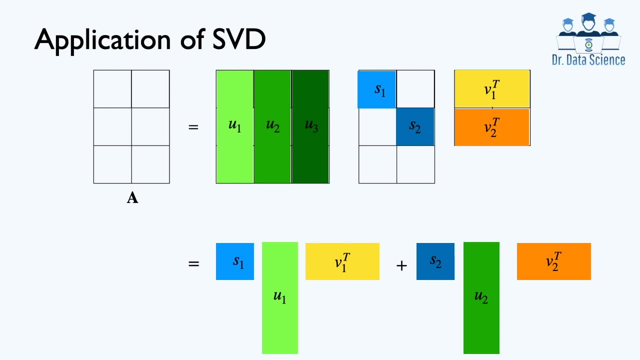 power of negative 16, and for us this is equivalent to 0.. so another question that we have: what is the application of svd? why is it so important? so let's go back to that example that we had originally. we have matrix a and then we have its singular value, decomposition, so we have the matrix u. 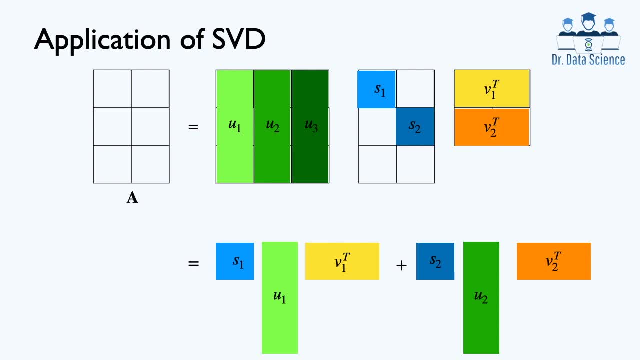 as three columns: u1, u2, u3, and then we have the singular values s1 and s2, and then we have the right singular vectors that we have them in the rows of uh, the matrix v. so now, using simple linear algebra operations, we can show that we can write this matrix a as the first singular value, which is: 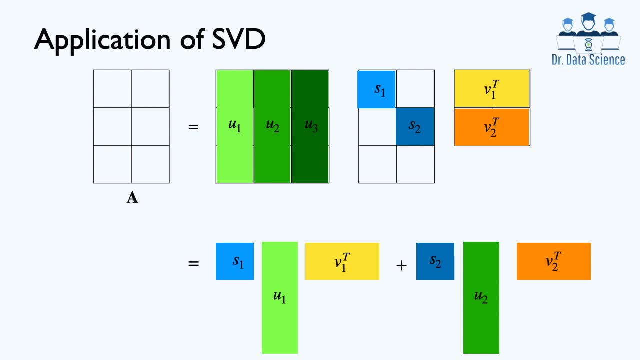 s1. and remember, s1 is just a scalar, it's a single number, so it's very easy to multiply it, and then we have the multiplication of the first column and then the first row, which is v1 transpose. so this is something that we call this a rank one matrix, because, if you're familiar, this is: 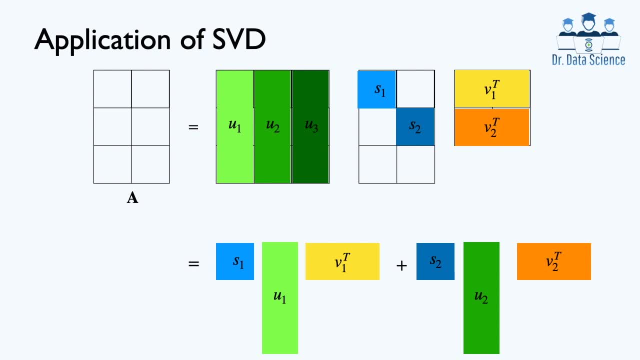 something that's called like outer product, right? so you have uh two vectors and then uh one of them here, for example, is m by one and the other one is one by n. so when you multiply you get something which is m by n, but it's a rank one matrix, and then you have the multiplication of the first column. 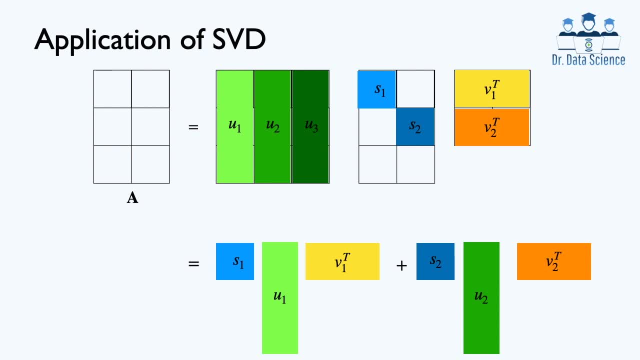 run out by decreasing m by m over here. so on th, if you take the sample out there, it's saying that m by n is equal thick, so m by n is random, right, and it's going to be another ordinary matrix, and that you just write downăm which is m by n, by m, as веч am quick, and you write a string. 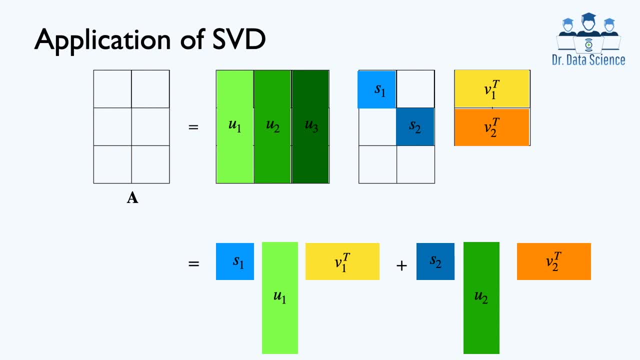 function of from in a linear matrix from. but then it says m is all zeros. so let's just write out m by n as this row there, this row and the next row. eight of these rows are all zeros and therefore m by n has the same ask, two, three zeros. so that means if you read this unit by n Sunday, we have 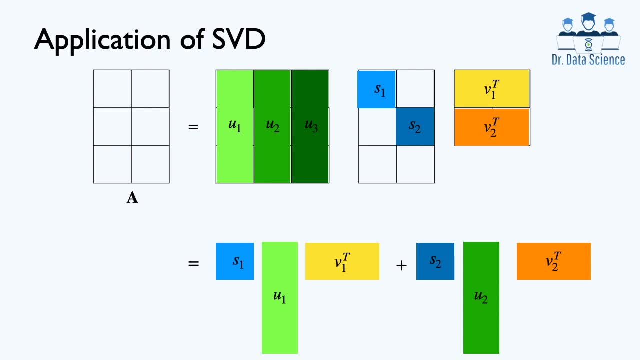 representing the matrix A And, if you want to go a little bit more in detail, that's something that we say- that this matrix is rank two because we only have S1 and S2, means that we have two non-zero singular values. 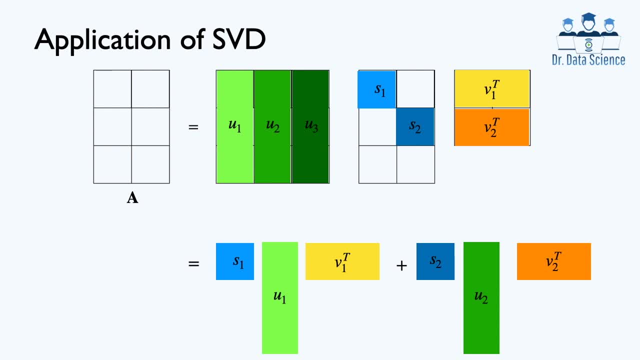 and this would be a rank two matrix. And the reason that this type of decomposition is very useful is that, let's say, you have done this singular value decomposition and you see that S1, the first singular value, is much greater than S2.. 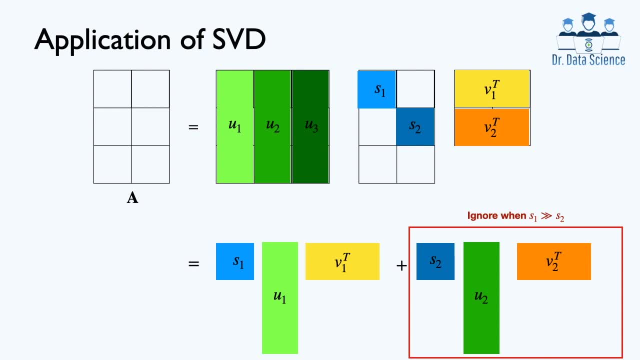 So this means that the first term is much more important than the second term. So if you need to reduce the redundancy in data or reduce the size of data, you can get rid of the second term and just approximate the matrix A using the first term. 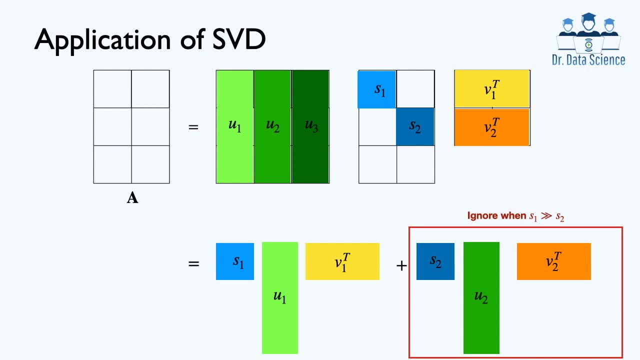 which is S1, U1 times V1 transpose, And that's what something that we call a low-rank approximation, which is very, very useful, And in recommendation systems, when you have huge matrices where, let's say, each row corresponds to different users. 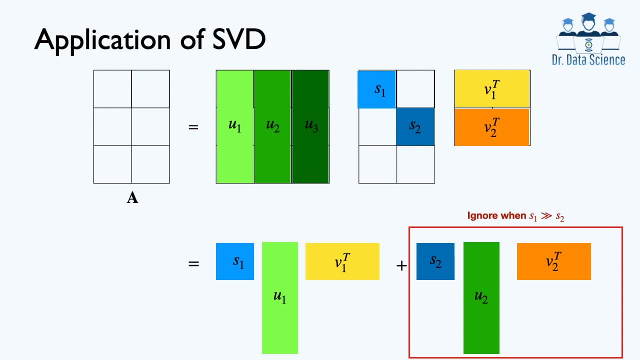 and each column refers to different items. there is definitely some kind of you know, some kind of structure or correlation in this matrix And this means that if you do singular value decomposition, you will have these type of decaying singular values that you can get rid of some of them. 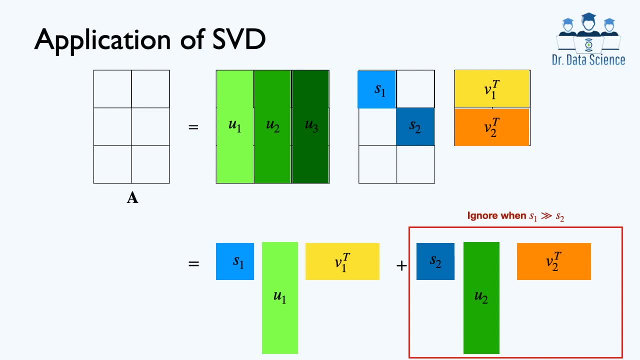 and these will allow you to extract more information from incomplete observations, Because what happens is that when you have a lot of items, a lot of users, for example, you can ask all users to rate all items in your database, So you need to be able to make predictions. 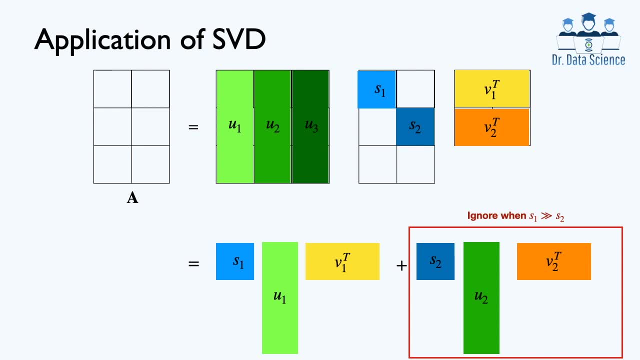 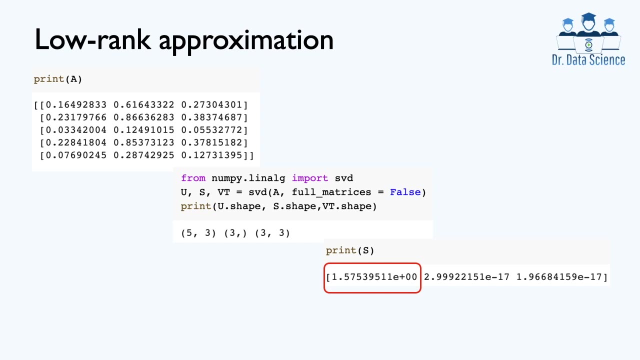 about the missing sort of like ratings And that's sort of like the basic idea here that you can use this type of low-rank approximation. And here what I've done to explain low-rank approximation, I've created this matrix A. 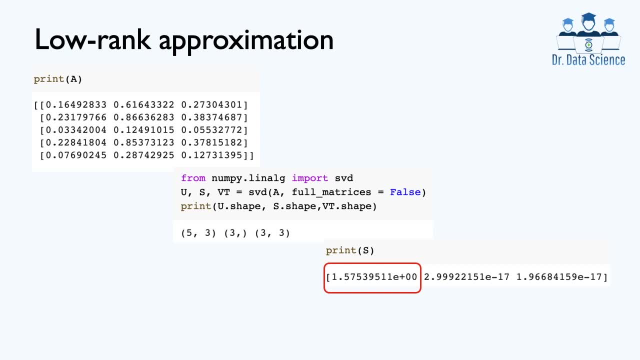 which has five rows and three columns. We import SVD And here what I'm doing is that I'm setting these full underscore matrices to be false. So if you look at the shape or the sort of like, the size of each of these singular vectors and singular values, 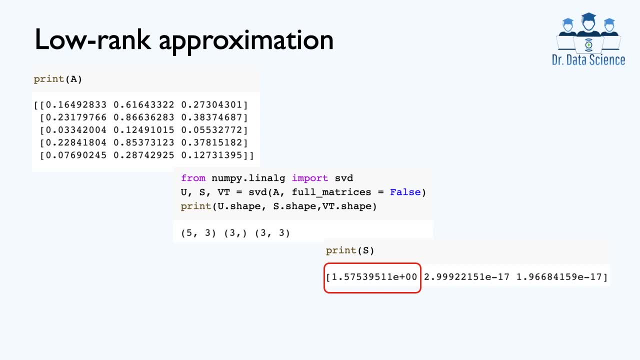 you can see that matrix U is five by three, So it's not any more square. And then the S is a one-dimensional array with three elements. You can also see the values of those three elements And then the matrix V transpose, which is, you call it here- VT. 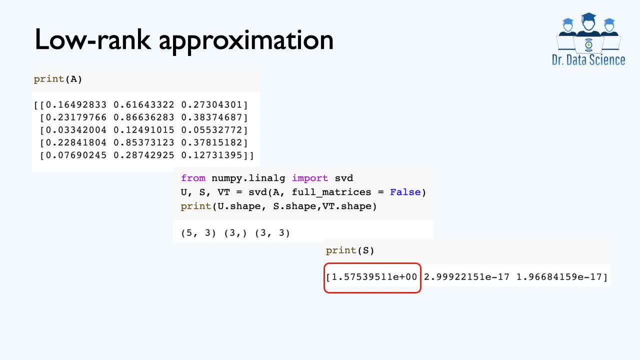 is also three by three, And here is exactly what we were talking about. If you look at S1, which is the first element of this one-dimensional array S, it's much greater than the rest, because the rest of them are like 10 to the power. 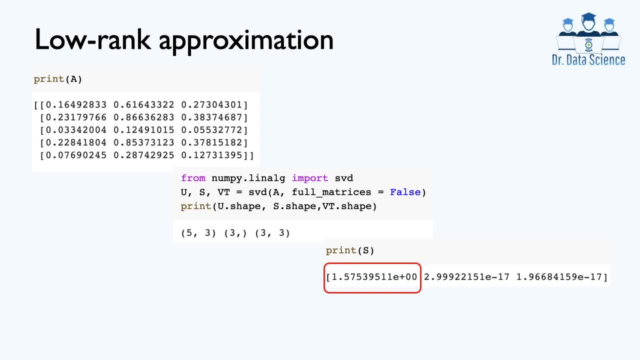 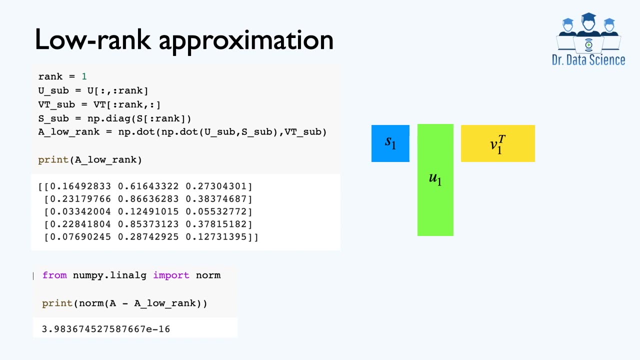 of negative 17.. So this means that we can just keep the first one and get rid of the other two singular values. And we can do so using this very simple technique that we have these matrices, U and V transpose, And we decide that the rank is one here. 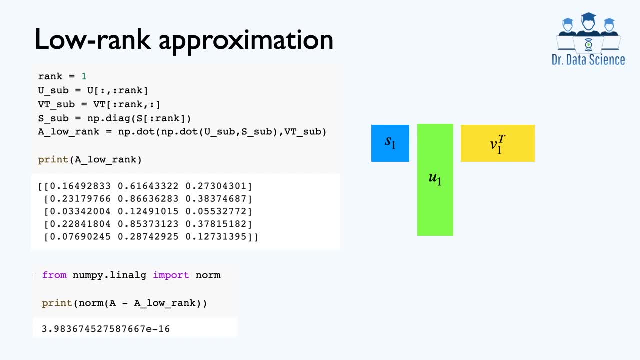 because, if we look at it, we only had one dominant or major singular value and so, because indexing starts from zero in python and numpy, we are gonna start from zero to one and one is excluding, so we are gonna just pick the first uh column of u, which is index at zero. 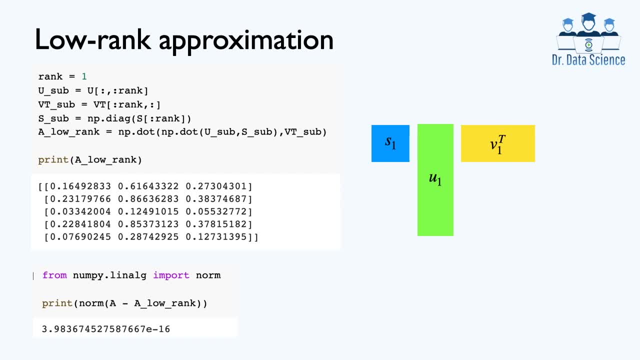 and similarly the first row of v transpose and also the first element in that one-dimensional array for uh single values, and then we can just multiply all these matrices together. instead of using that multi dot function here i'm using np dot dot. so this is just when you want to. 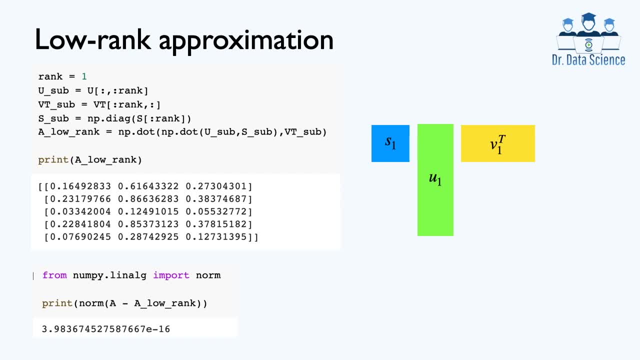 multiply two matrices. that's why i'm gonna first multiply u and s and then i multiply the result of this by v, and when we do this multiplication now we have this approximate version- that's why i call it a low rank- and we can again find the difference between the original matrix a and a low rank. 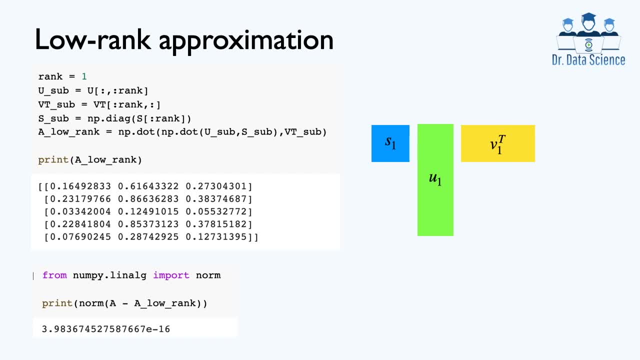 and we can see this is in the order of 10 to the power of negative 16, which, again this is almost zero. so this means that we have a perfect reconstruction of matrix a using this very simple formula, that we have one singular value, one column vector times one row vector. 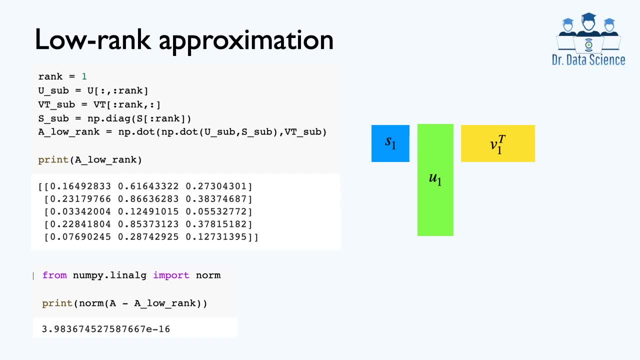 so you can see that now, instead of saving all those five by three, which would be 15 elements in the matrix a, we can just save all these entries for u1 and v1. so we have five elements in u1, three elements in v1 and also one singular value. so we have some type of data compression. so that's for the 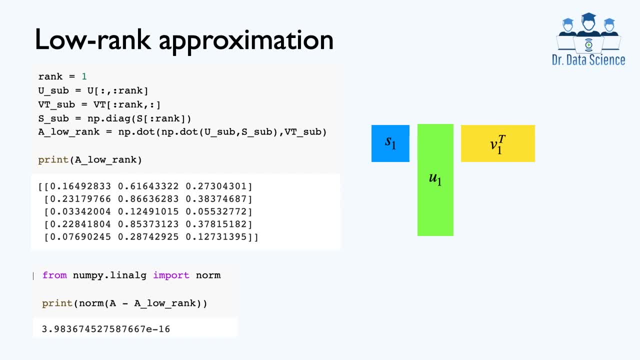 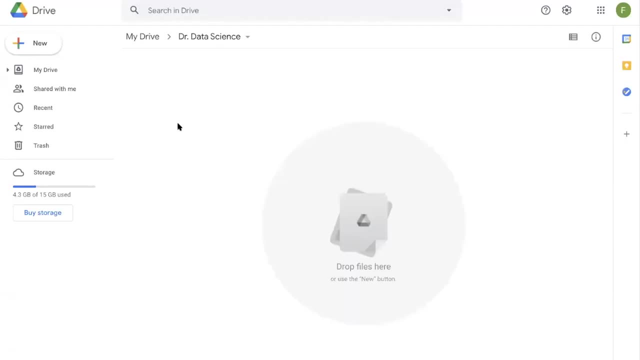 lecture, part of this um video, and then we're gonna have a step-by-step implementation in google cloud. see you soon. okay, now let's have a step-by-step implementation of these in python using google cloud, as we discussed before. the first thing you need to do is that you need to go to google. 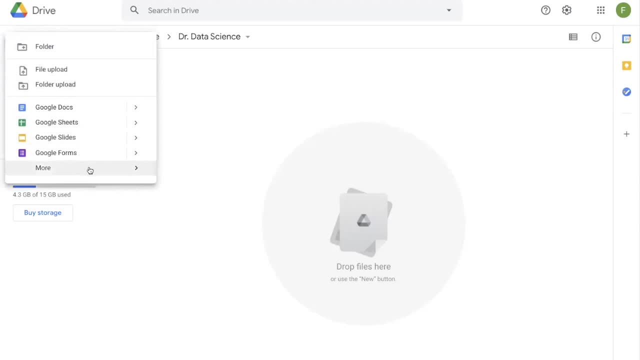 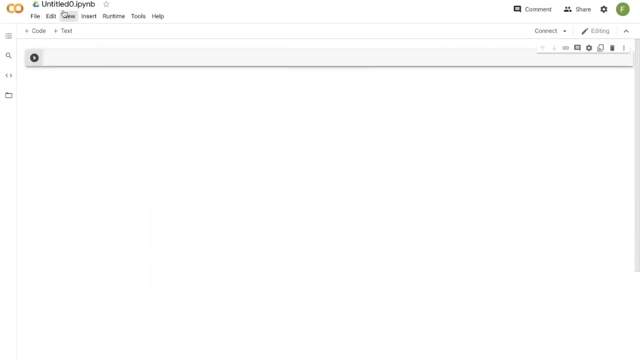 drive drive- google drive- drivegooglecom, and then create new. and if you have already created a new, created a Google Cloud file, you can find it here. Otherwise, you use connect more apps. So here we used to Google Collaboratory or Google Cloud, And the first thing you want to do 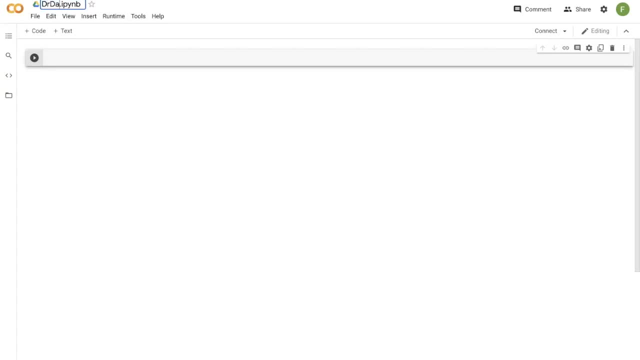 you can change the name of your Jupyter notebook. We call this Dr Data Science for obvious reasons- And then you start with importing modules that you want. So here we are going to start with importing NumPy, And also because we are using singular value decomposition from NumPyLinOut. 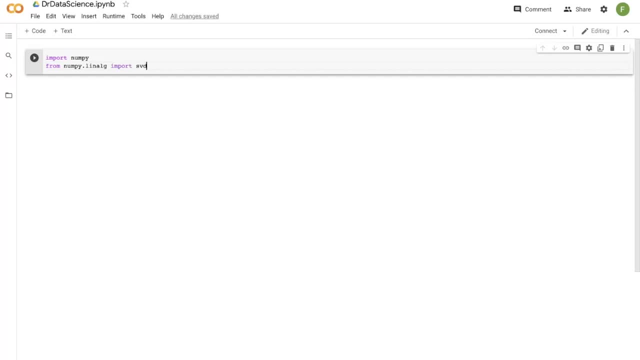 we are going to import SVD. So now we run this cell And now we can create the two-dimensional array that we had in the lecture. So we use nparray And now we give a list of the rows that we have. So the first row was 1 and negative 0.8.. 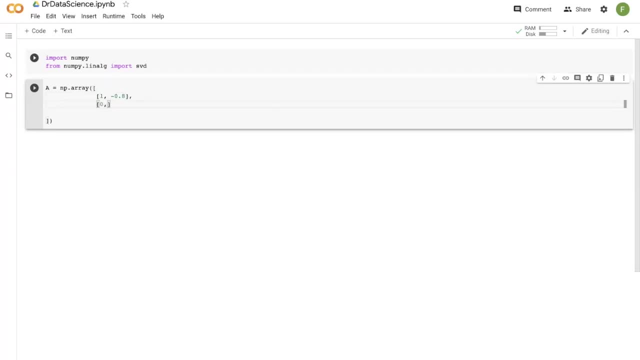 The second row was 0 and 1.. And then the third row is 1 and 0.. So if I run this, we see that we get an error message which is basically saying that np is not defined And that's because we didn't use import NumPy as np. I use this because I want to show you that. 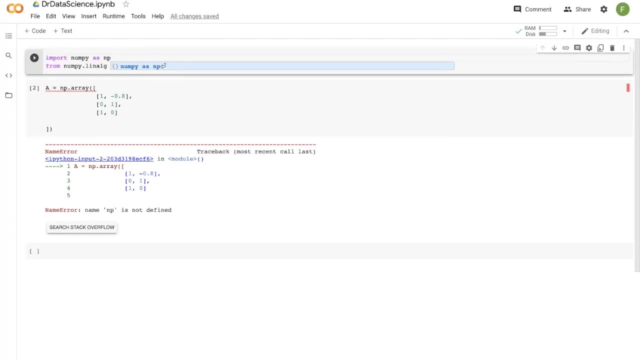 how easy it is to get the error messages. But the good thing about Python in general is that it's usually easy to find out the main cause of the problem. So here we are going to import NumPy as np And the other one for SVD looks good. So now we run this And this time we don't have any error. 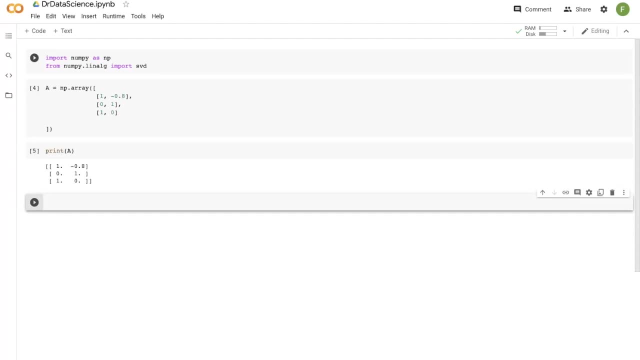 message. So now we can use printA And we can see that now we have this two-dimensional array, We can also use dot shape to find the number of rows and columns. So obviously here we have three rows and two columns. Now in order to find the single value decomposition. 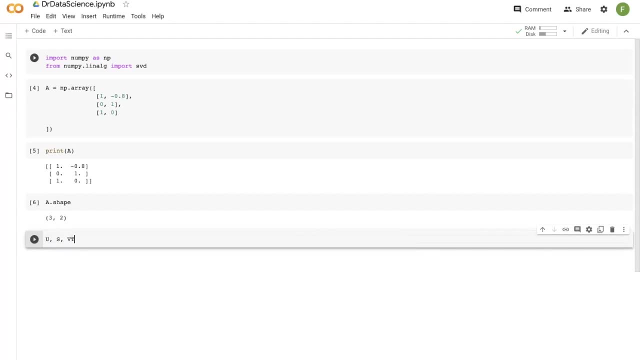 we use u, s and then v transpose. That's the notation that we had, But I just call this vt. So this is the transpose, the matrix v. This is just the name, so that I remember that this is the transpose of v, not the v itself. And now we use st. 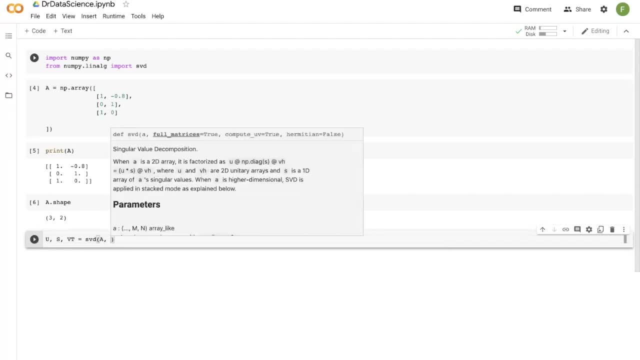 vd. The first option is to give the two-dimensional array that we have, And that's what I like about using Google Cloud. So you can see that here, all the instructions that we had in the documentation page. So let's say, put full matrices equal to true. 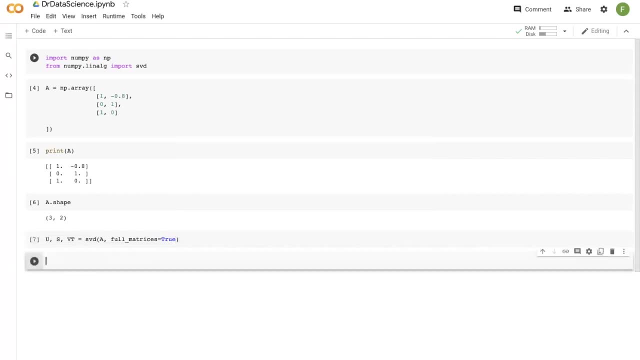 So this is the default option, And if I do so now, I can look at the shape of these three rows, and these rows are the same. Having seen how simple that looks, we can hide this unit in another point of time, One of the farthest options where you can look. 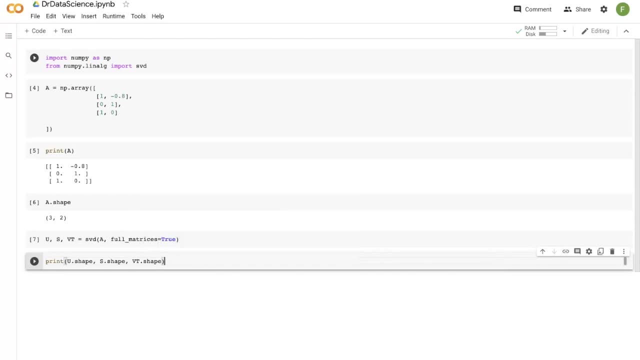 is in the Point ну dimensional array with two elements. So you can see here the difference between a two-dimensional array and a one-dimensional array. When you have two-dimensional array you have two numbers, So you have a two-pole, for example like three comma three. But when you have a one-dimensional array, 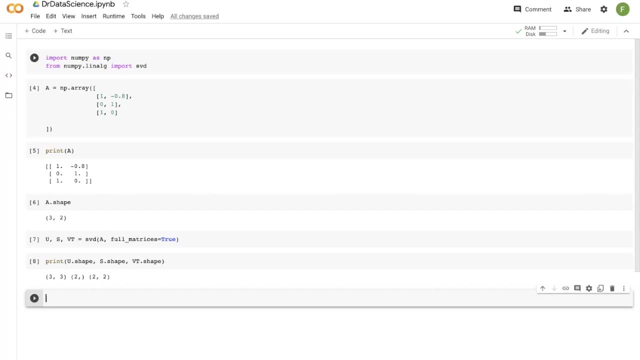 you have two comma and then there's nothing there. So that means that S is a one-dimensional array. And then we have this matrix VT, which is two by two, which is a square. Now we can write the same thing, but this time I'm going to set four. 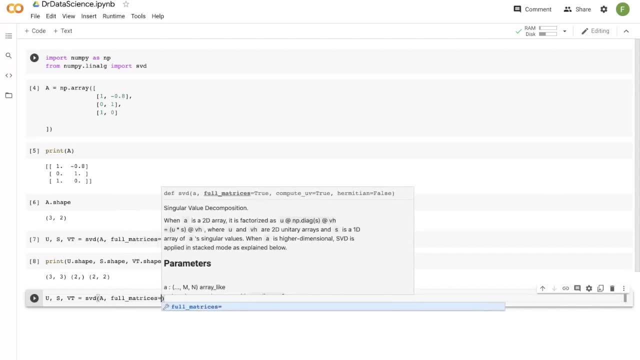 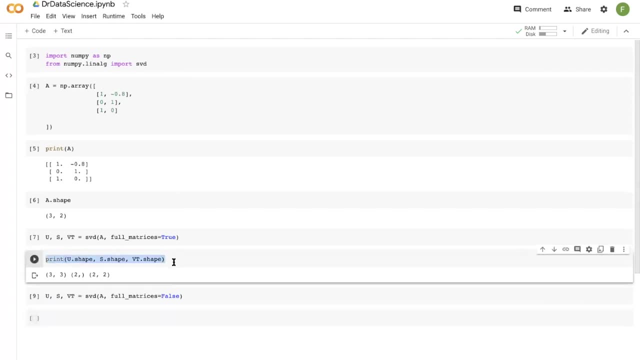 matrices to be false And we can just copy paste the previous line to see the difference in terms of the number of rows and columns, As we discussed in the lecture, because now the variable S has only two elements, So this means that the last column of U is not useful. 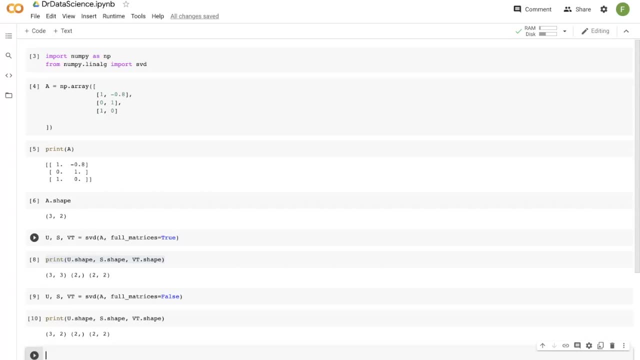 So that's why when you set four matrices to be false, now we automatically get rid of that column. So now the matrix U is three by two and S is a one dimensional array with two elements, and VT is also two by two, And now we can also look at the elements. 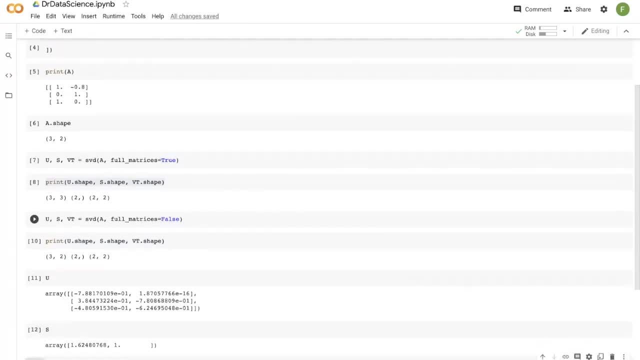 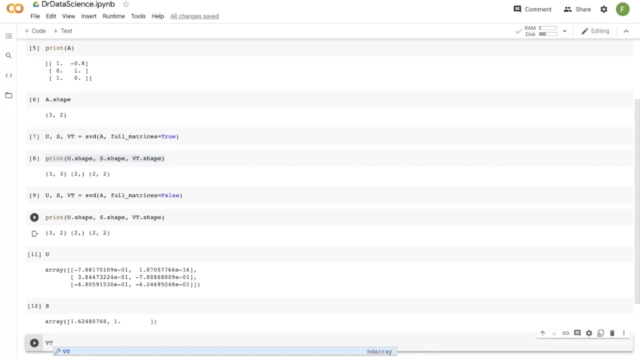 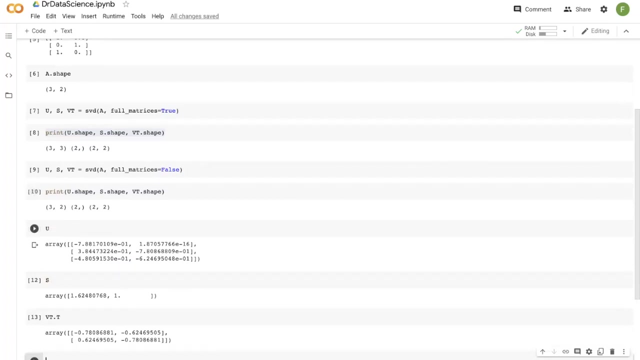 that we have here, We have U, we have S. that's our one dimensional array. And then if you want to have the right singular vectors in columns, we can use dot transpose, that I can use this option, or you can use NP dot transpose. 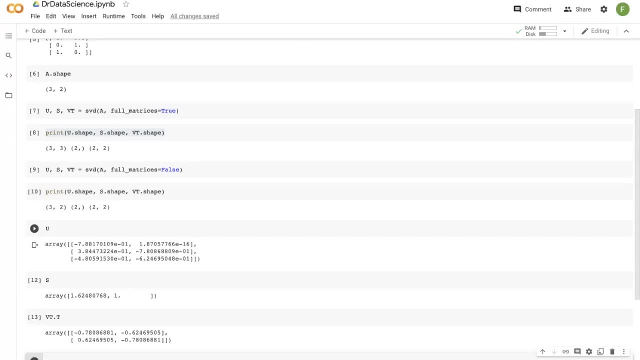 And this summarizes the main steps that you have to take to find the singular value decomposition. It's relatively straightforward: You need just from numpylinux and import SVD. And then the very important option here is that, whether this full underscore matrices is true or false,